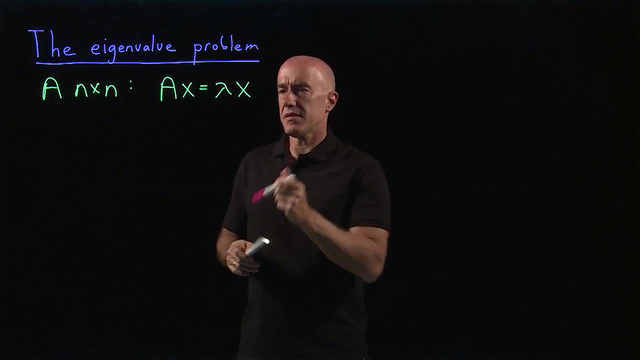 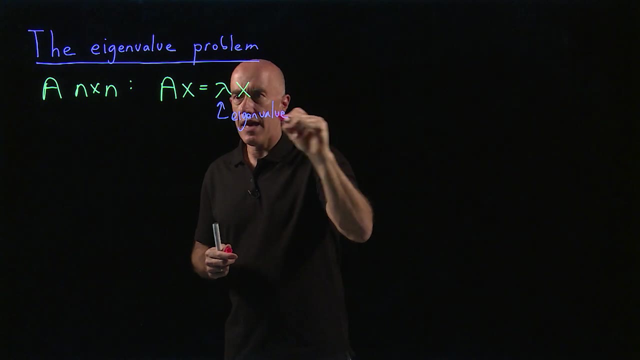 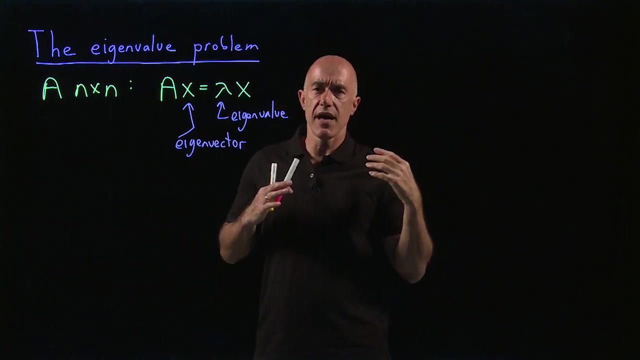 multiply it by a number lambda. This lambda is what we call the eigenvalue and this x is what we call the eigenvector. OK, So for each eigenvalue you have an associated eigenvector. So the eigenvalue problem is that, given a n by n, matrix A. 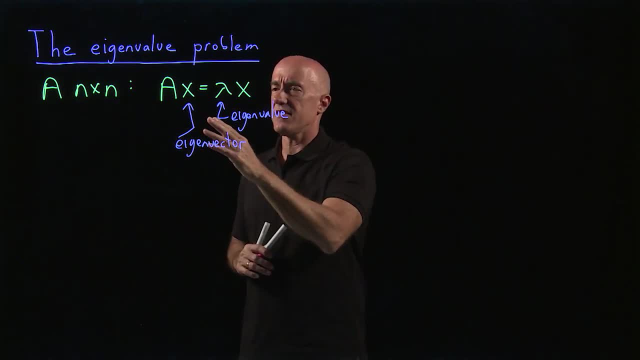 you want to find its eigenvalues and its eigenvectors. So those are the scalars and the vectors that can satisfy this equation. In this video, we're going to try and show you how to solve this problem, and I will find the eigenvalues. 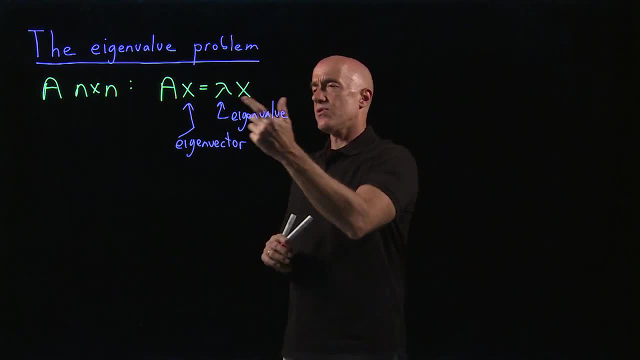 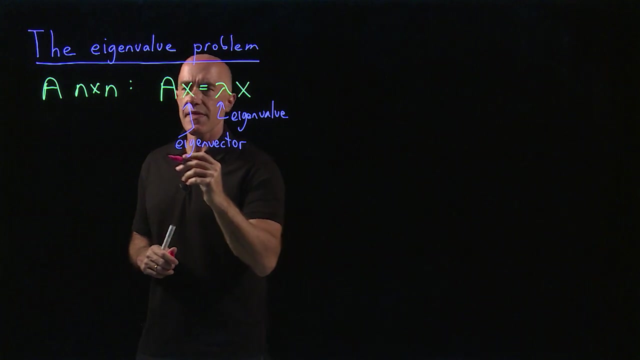 at least for a 2 by 2 matrix. So how do you tackle this problem? A is n by n matrix, So the way to do this is to introduce an n by n matrix on the right-hand side of this equation also. It's not that hard to do. 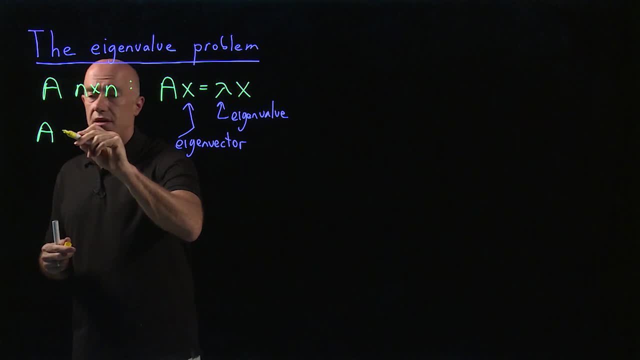 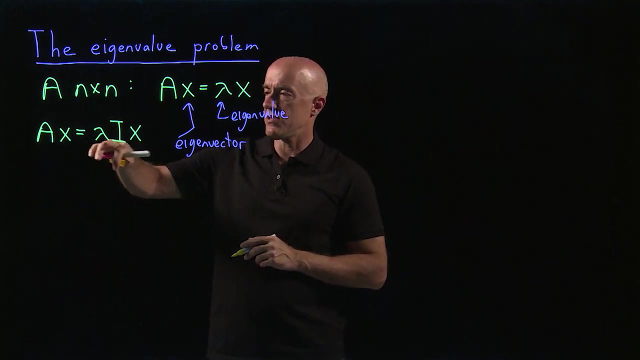 All we need to do is introduce the identity matrix, so Ax equals lambda, And then we sneak in an n by n identity matrix onto the right-hand side. So now we have an n by n matrix times a column vector x equals an n by n matrix. 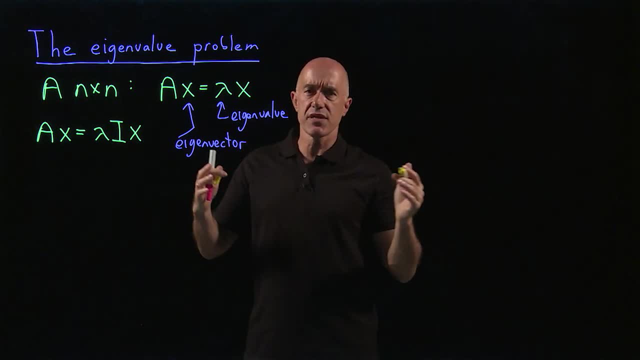 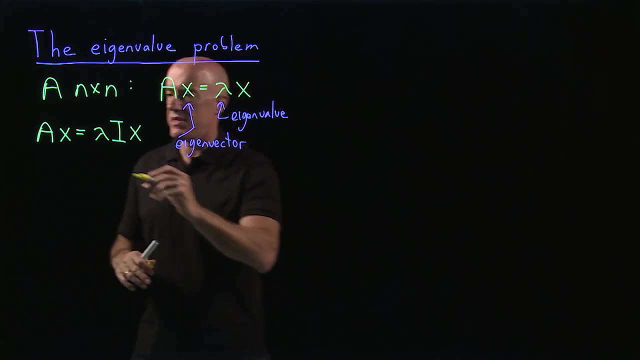 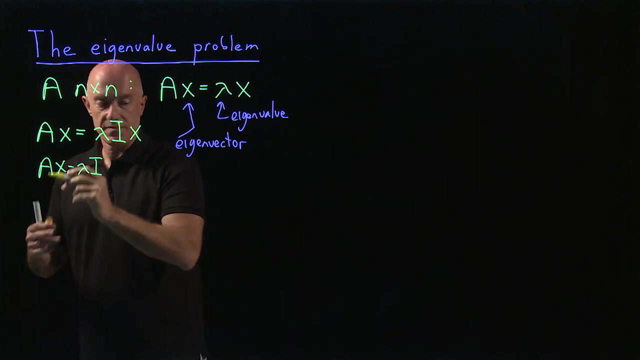 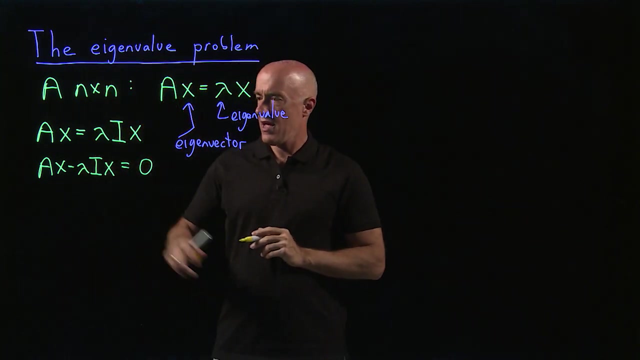 Lambda i is just a matrix with lambda going down the diagonals times another column vector. So we can regroup the terms here and we can write: Ax minus lambda i, x equals 0. That's fine And then we can factor out the x. 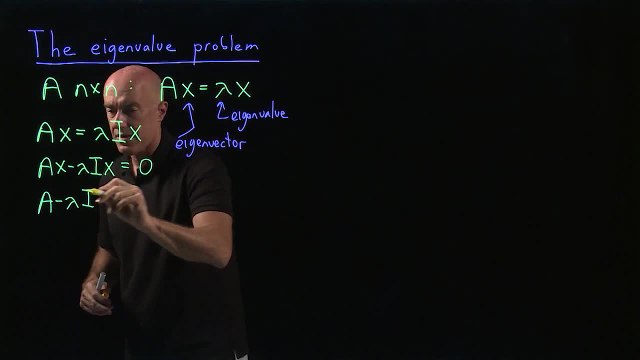 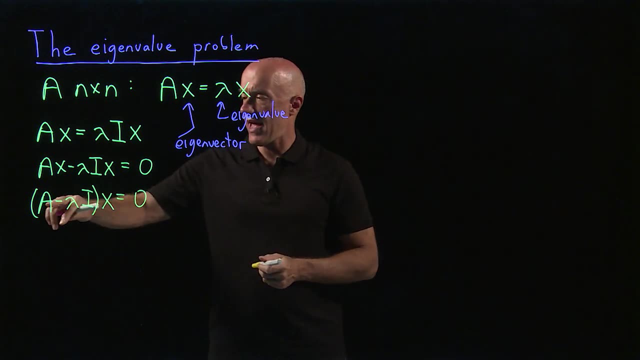 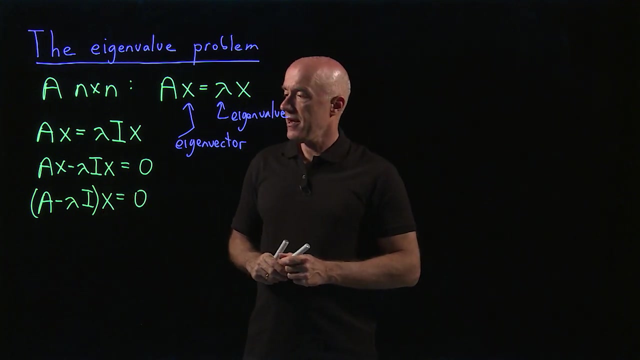 So then we can finally write: A minus lambda i times x equals 0.. So now we have an n by n matrix times an n by 1 column vector equals 0.. OK, We just learned about determinants. We know that if the determinant of A minus lambda i was not 0,. 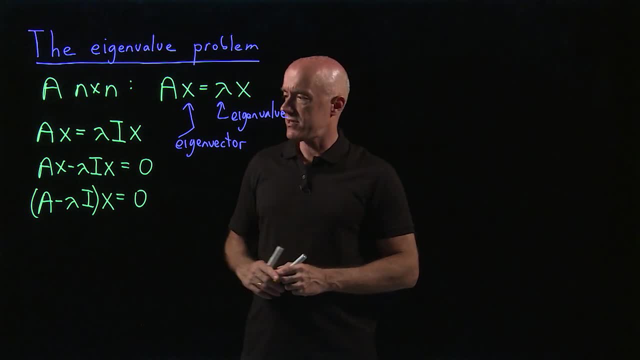 then A minus lambda, i would have an inverse matrix And then we can multiply on the left by the inverse and then we would get x equals 0. x equals 0 is always a solution of Ax equals lambda x And that's called the trivial solution because it 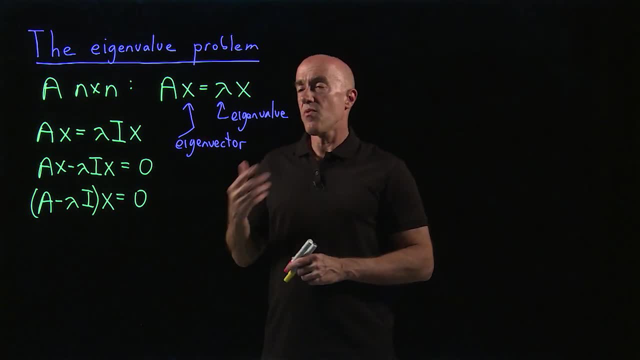 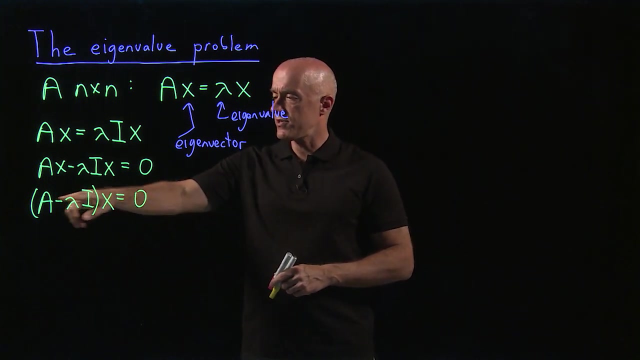 doesn't really tell us what we want to know. What we want to know are the values of lambda and the vectors x that satisfy this equation, where the vectors x are not just the 0 vectors, They're something other than 0. So in order for this to have a solution other than x equals 0,. 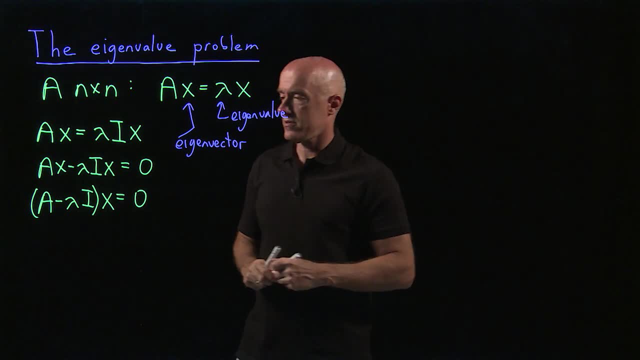 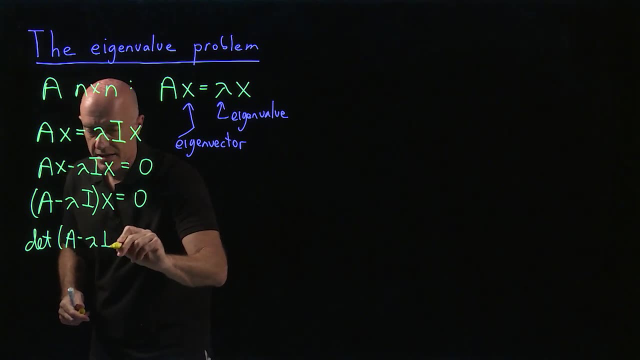 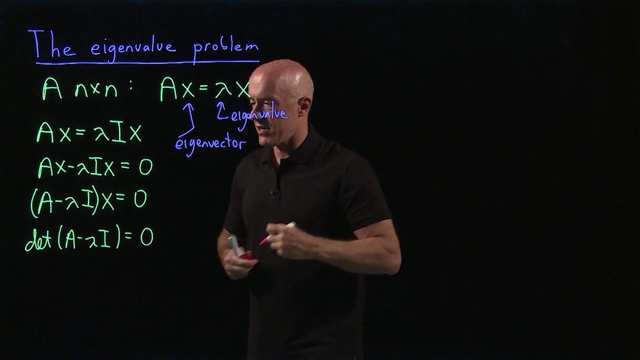 the determinant of this matrix has to be 0.. OK, This cannot be an invertible matrix. So the determinant of A minus lambda i equals 0, OK, minus lambda i has to be 0.. That's the equation for the eigenvalue lambda. 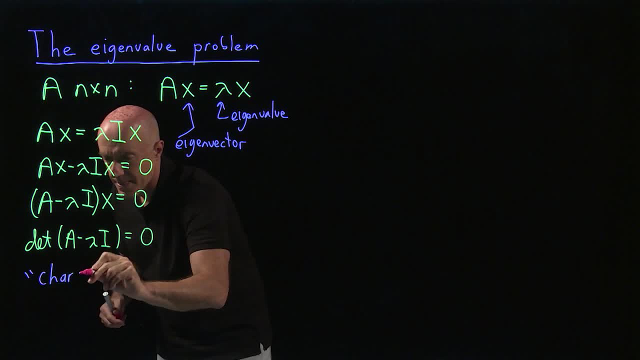 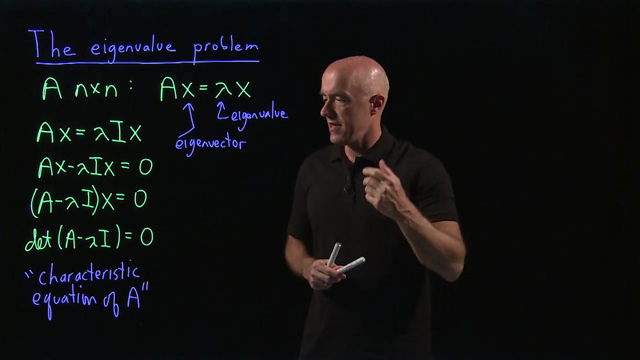 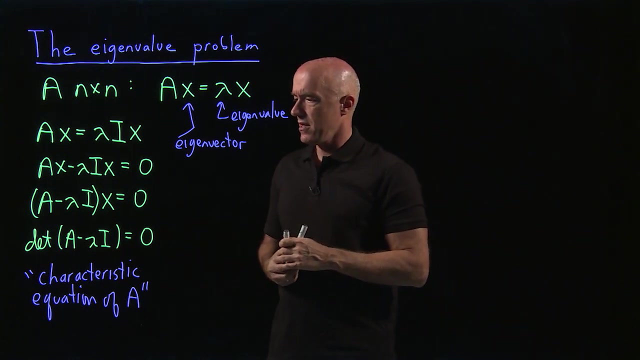 That's called the characteristic equation of the matrix A. That's the fundamental equation in the eigenvalue problem. What is the characteristic equation? What type of equation is it? We know the determinant of an n by n matrix. You can calculate that. 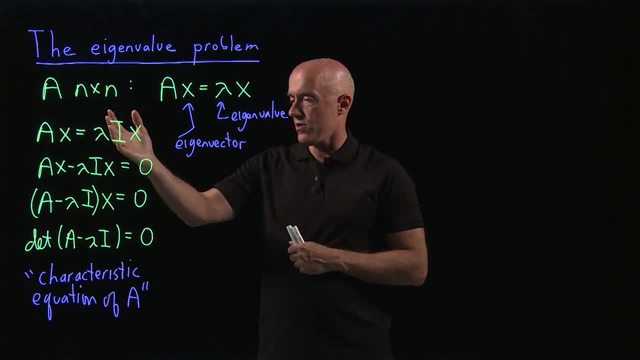 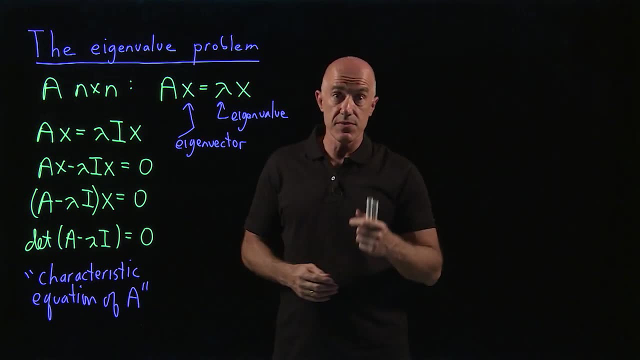 You need to take an element from the first row and multiply it by an element in the second row and an element in the third row, And then you have all these terms, But you always have, And each, Each row. you have a lambda right. 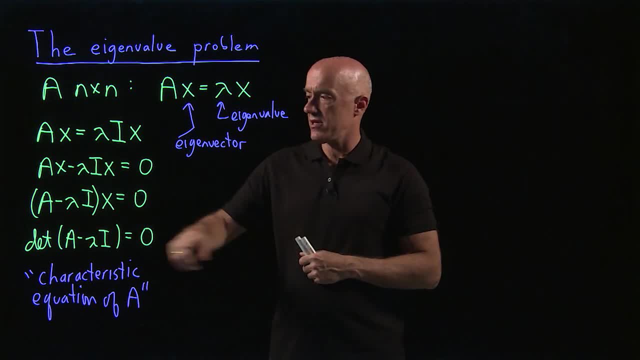 So the first row along the diagonal is A11 minus lambda. The second row at the diagonal is A22 minus lambda. So each row has a lambda in it. So when you construct you do the expansion to get the determinant of A minus lambda. i. 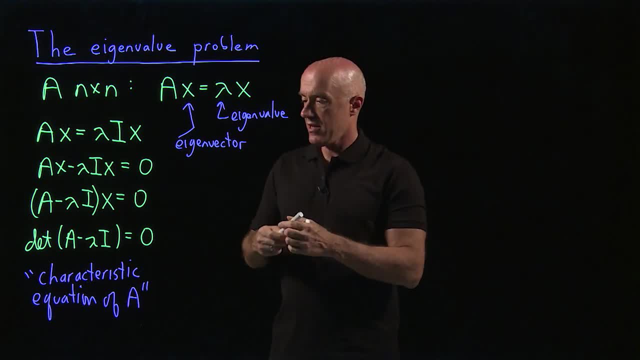 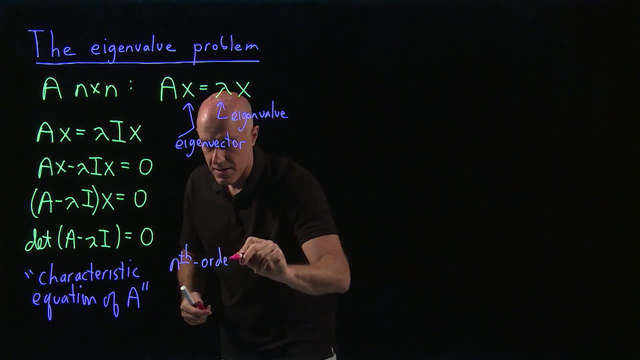 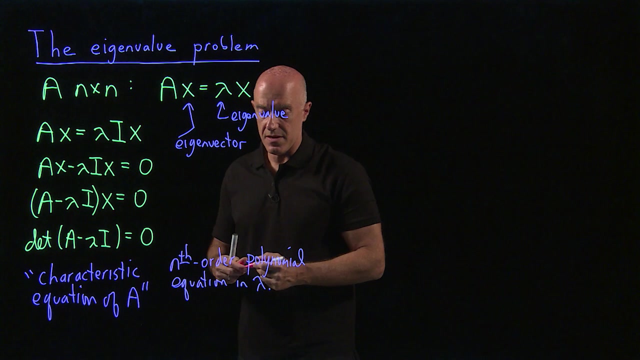 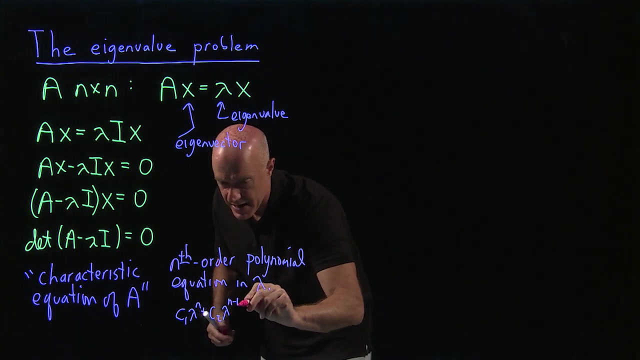 you end up with a polynomial equation in lambda. So in fact this is a nth order, Because A is n by n. This is an nth order polynomial equation in lambda. OK, What is a polynomial equation, right? So C1 lambda to the nth plus C2 lambda to the nth minus 1 plus. 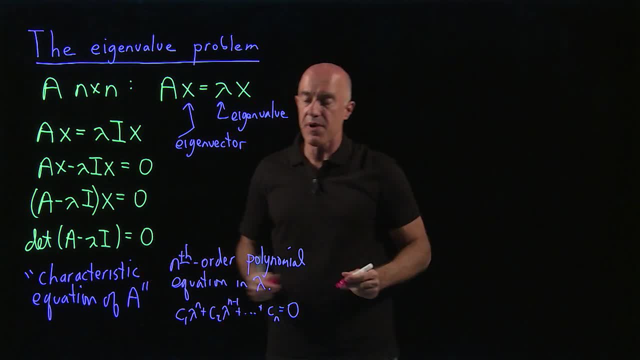 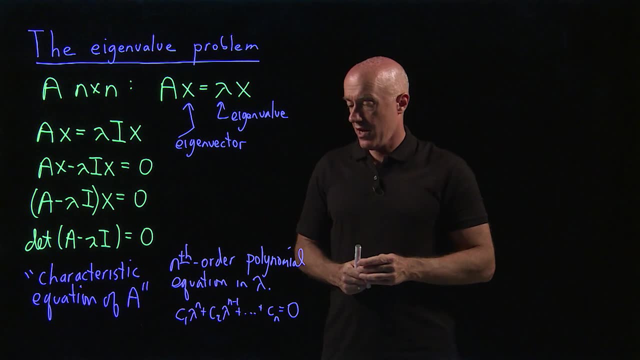 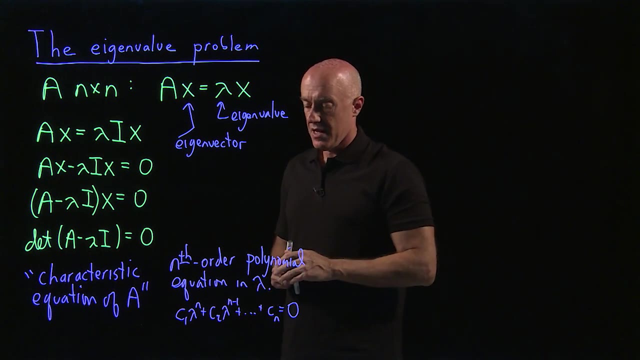 Cn equals lambda Equal to 0. That's a polynomial equation. OK, These polynomial equations have roots. They're in fact n roots. if you include the concept that roots can be repeated, The roots can be real, The roots can be complex. 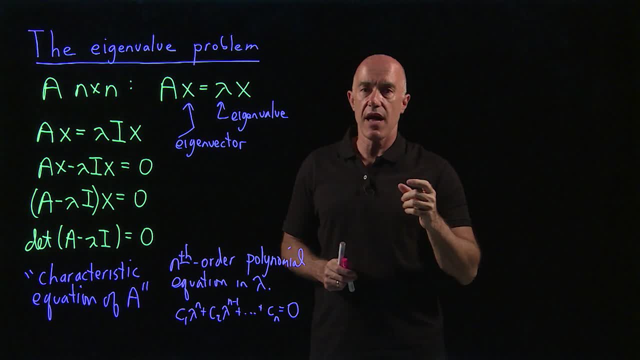 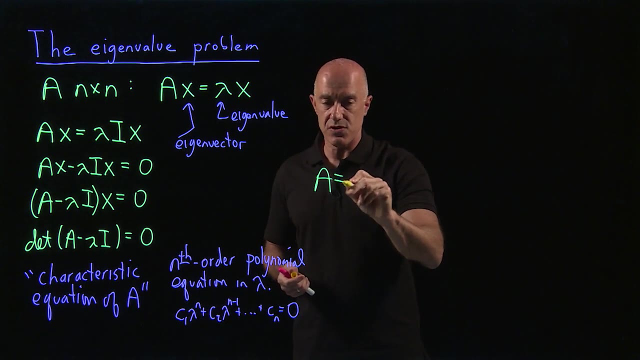 So we can in the rest of this lecture. I can show you an example. We can consider a general 2 by 2 matrix And try to compute the eigenvalues of that matrix. So let's start with a general 2 by 2 matrix. 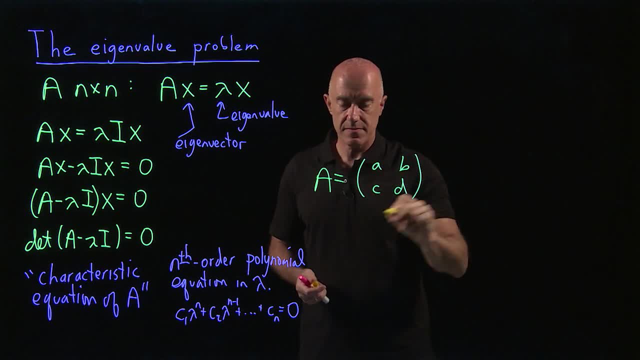 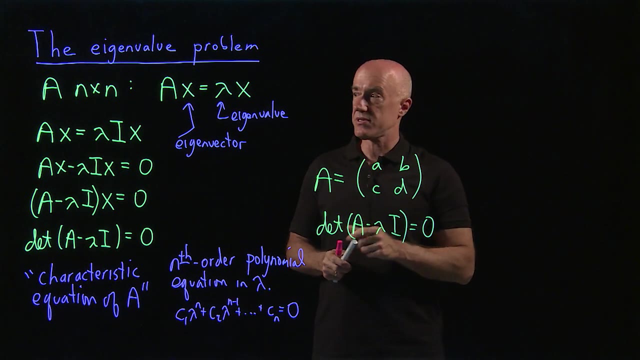 A, B, C, D, And we try to compute the determinant of A minus lambda i, equal to 0.. So the characteristic equation of a general 2 by 2 matrix. So you see how the eigenvalues come out In the simple case of 2 by 2.. 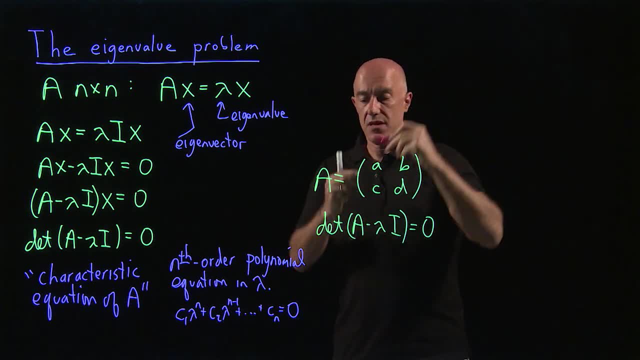 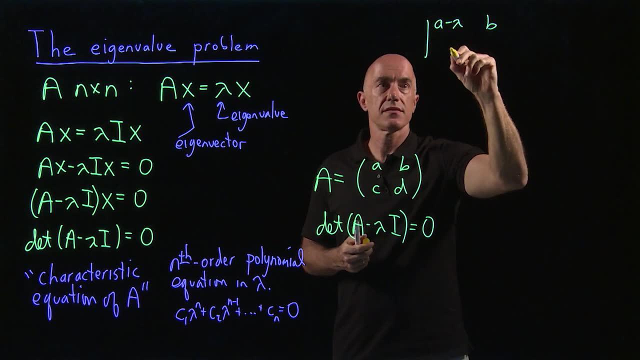 So determinant of A minus lambda i equals 0. That one looks like A minus lambda, B, C, D minus lambda. So the determinant of this 2 by 2 matrix, We know how to do the determinant of 2 by 2 matrices. 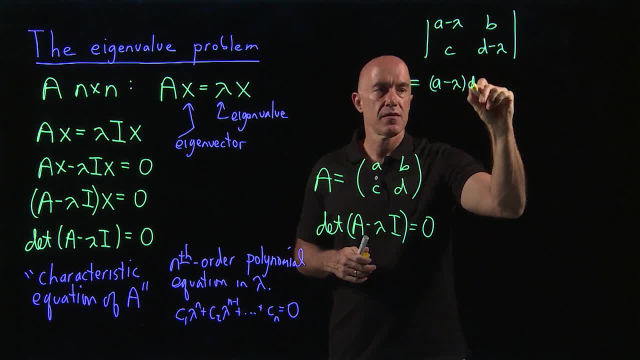 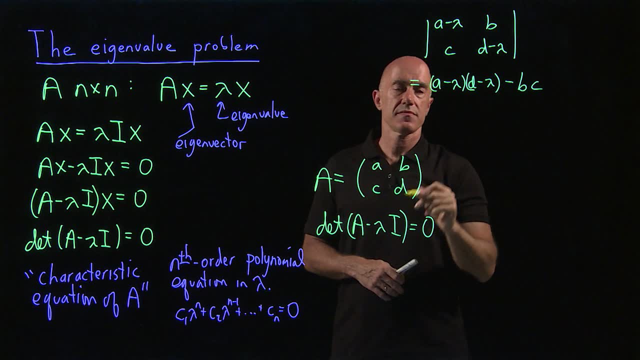 This is A minus lambda times D minus lambda. OK, Minus lambda Right The diagonal, minus B C. We can expand this quadratic. So minus lambda times minus lambda is lambda squared. Minus A lambda minus D lambda is minus A plus D lambda. 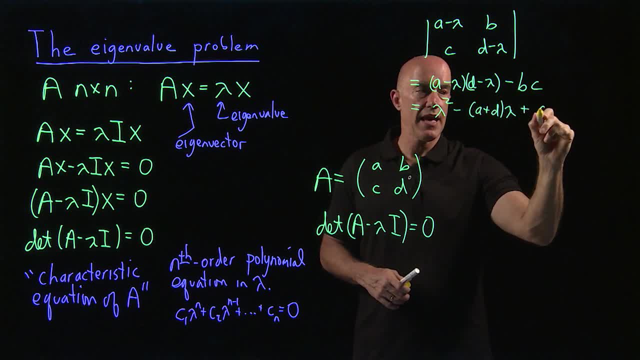 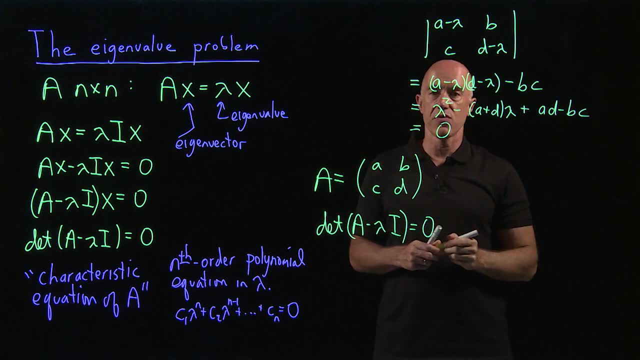 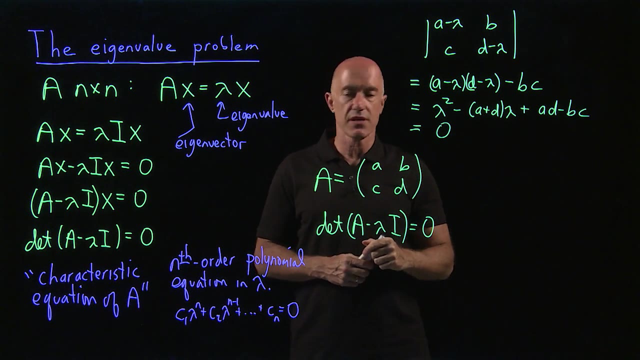 And then A D minus B C is plus A D minus B C, And that's supposed to be 0.. That's the characteristic equation. OK, This is in general the characteristic equation for a 2 by 2 matrix. 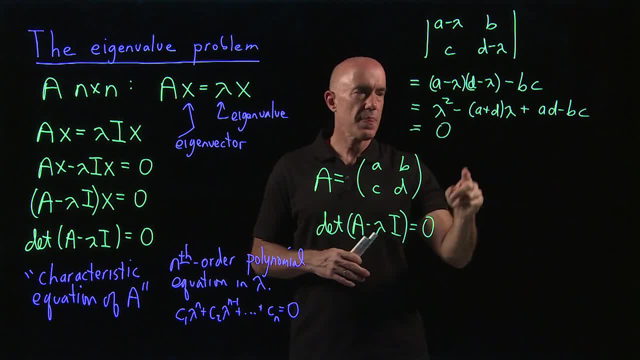 Just for your information, this A plus D term is the sum of the diagonal elements of the matrix A That has a name That's called the trace of A, And the A, D minus B, C term is the determinant of the matrix. 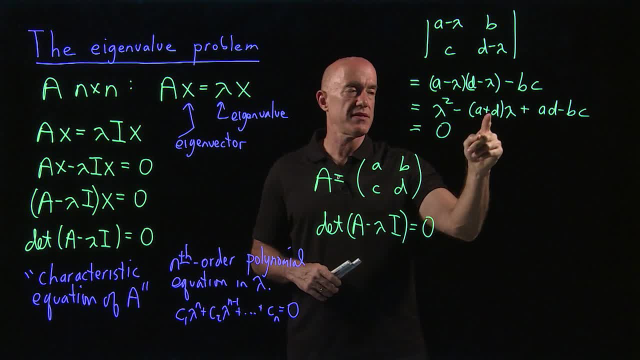 So this is lambda squared minus trace of lambda, plus determinant equals 0.. That's a general form for a 2 by 2 matrix. But it doesn't really matter, You can just remember how to calculate. OK, So for the eigenvalue problem for a 2 by 2 matrix, 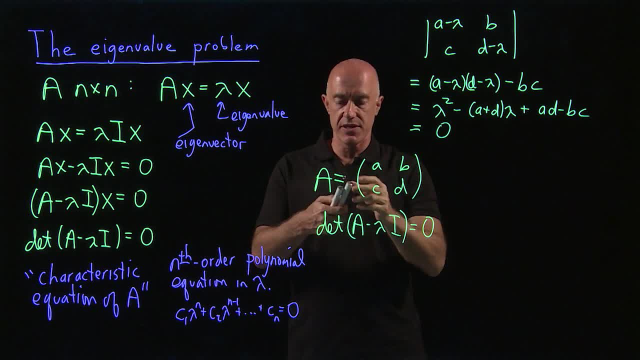 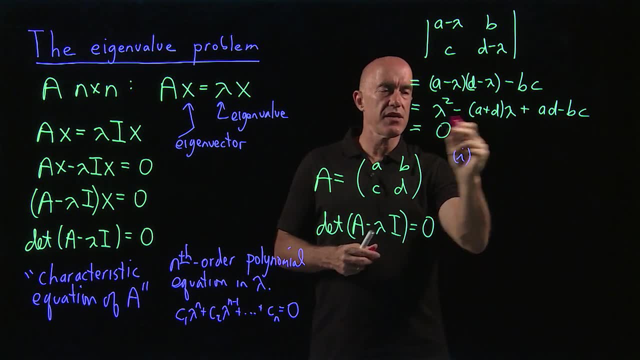 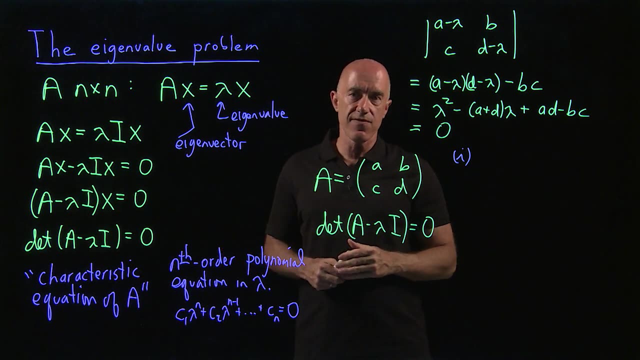 the eigenvalues are a solution of this quadratic equation. And then there are three possibilities: Yes, Yes, Yes, Yes, Yes, Yes. So the quadratic equation right, ax squared plus bx plus c equals 0, has the quadratic formula: 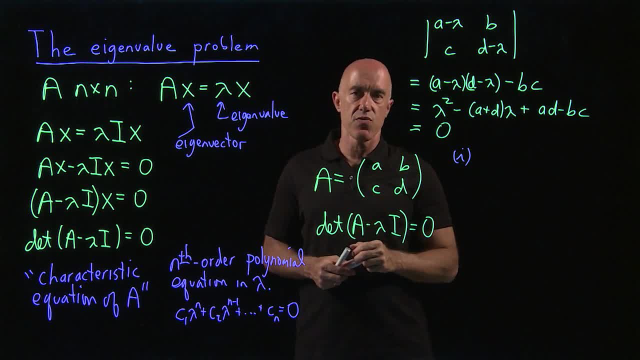 as the roots Negative b plus or minus, the square root of b squared minus 4ac over 2a. Everybody learns that in secondary school, in high school. But for a quadratic equation that b squared minus 4ac could be positive. 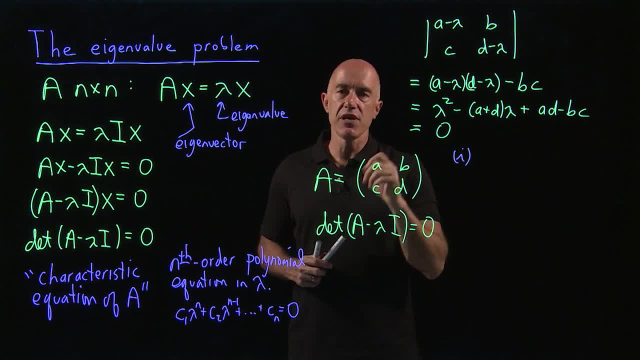 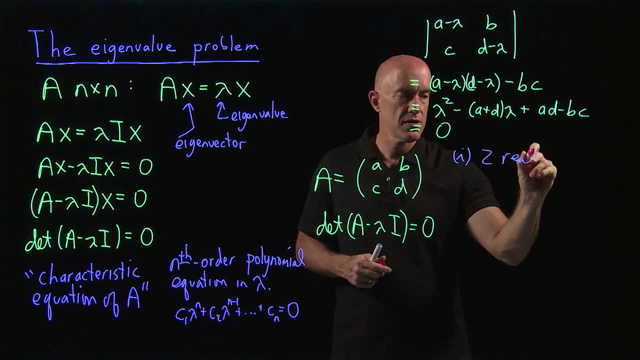 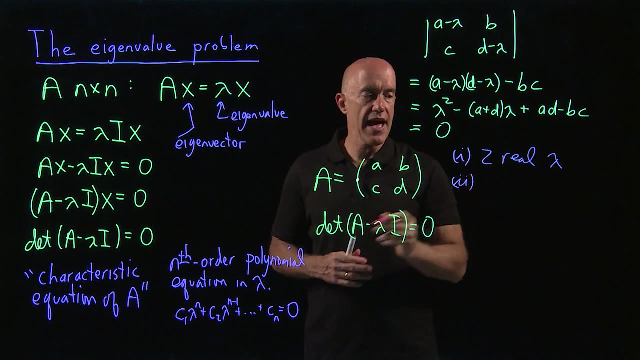 it could be negative, or it could be 0.. zero. so you have three possibilities for a quadratic equation. You can have two real values of lambda, so two real eigenvalues, or you can have b squared minus 4ac, negative, and then you take the square root of a negative number, so you can 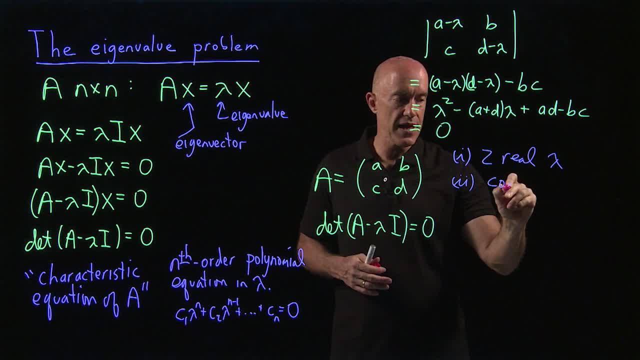 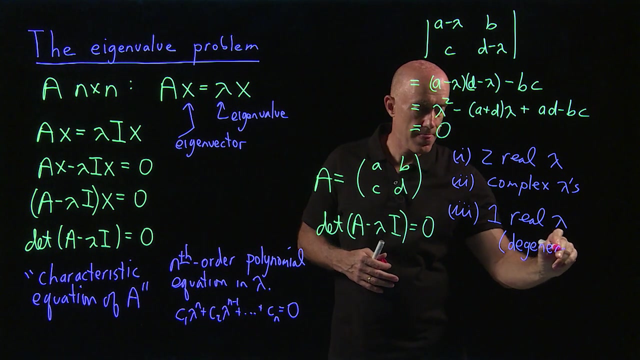 have complex eigenvalues, so complex lambdas. And then the third case would be: b squared minus 4ac equals 0, so then you only have one real lambda, So that one has a word. we say that the eigenvalues are degenerate. okay.